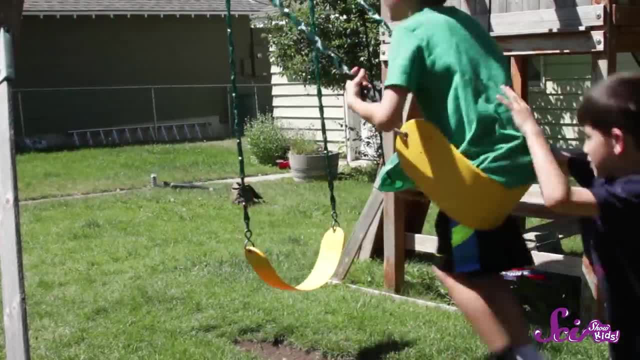 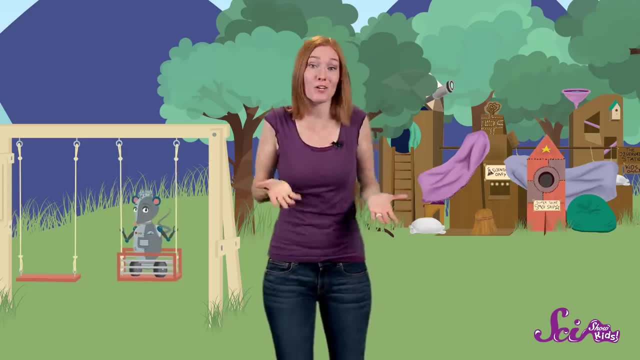 a swing, he's putting a force on you which makes you and the swing move. Or maybe you're swinging by yourself. When you pump your legs, that movement puts a force on the swing too. But unless you or your friend or something else puts a force on the. 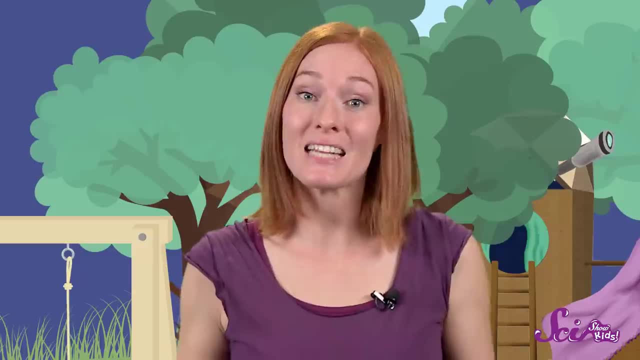 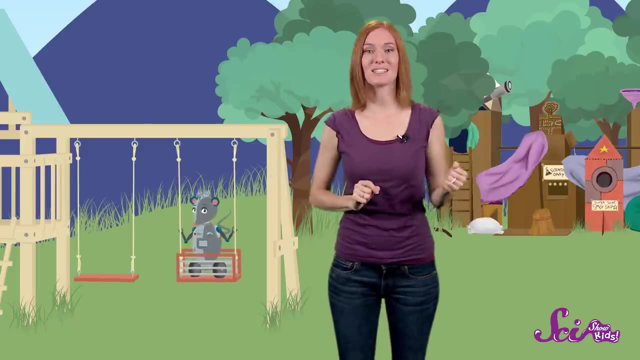 swing, it's just going to sit there. That's part of what Newton figured out. Now remember the second part of Newton's rule. It says that when something is moving, it'll keep moving unless something makes it stop. So does that mean that when something is moving, it'll keep moving unless something 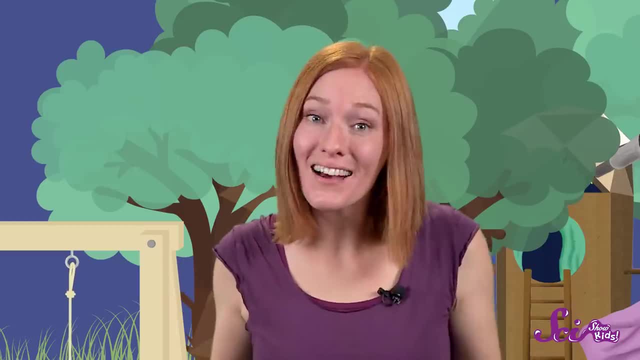 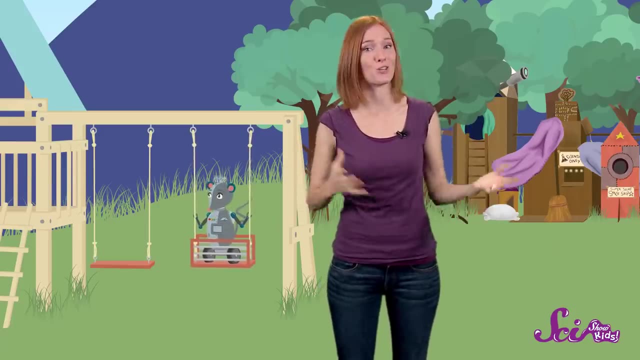 makes it stop And once you get going on the swing, you'll keep swinging forever. Well, I gotta say that sounds pretty awesome, But it can't happen, Because when you're on the swings there are forces around you that will make you stop moving. 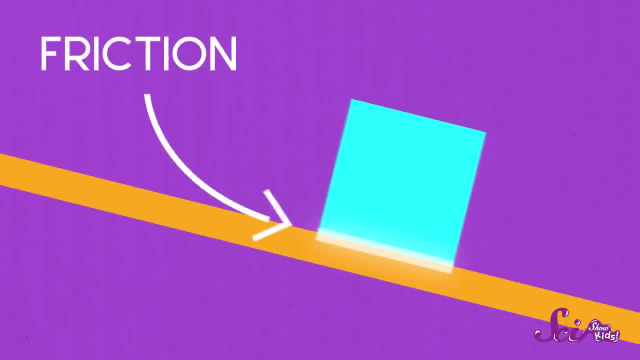 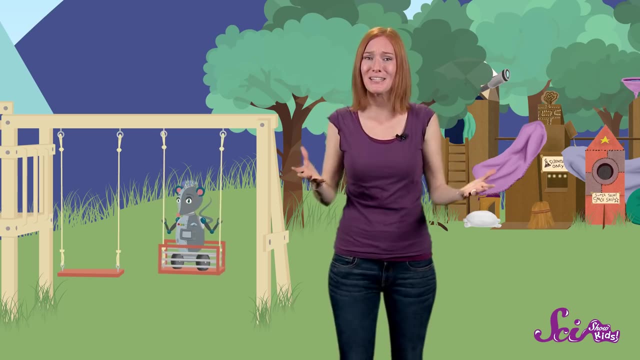 One of the main forces is friction. Friction is the force that happens when two things rub against each other, And I bet you've seen how it works before. Imagine you've been swinging for a while, pumping your legs until you got good and high, and then you. 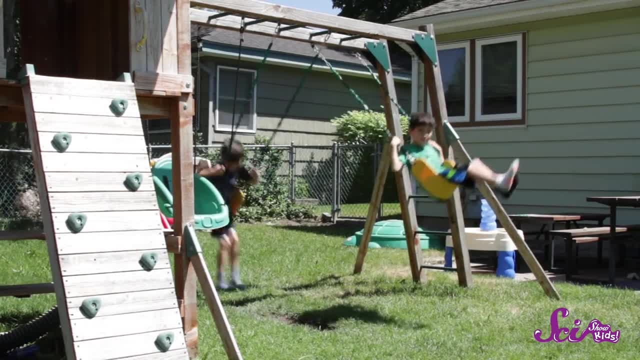 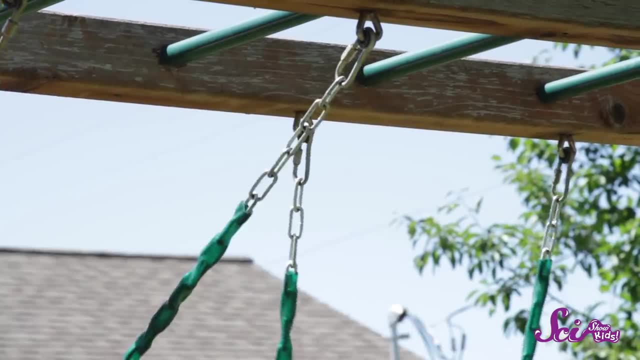 stop pumping. As you keep swinging back and forth, there's a lot of friction between you and the air, And there's also friction where the swing's chains meet, the top of the swing set Together. all of this friction makes you slow down, And if you wait long enough, you'll come. 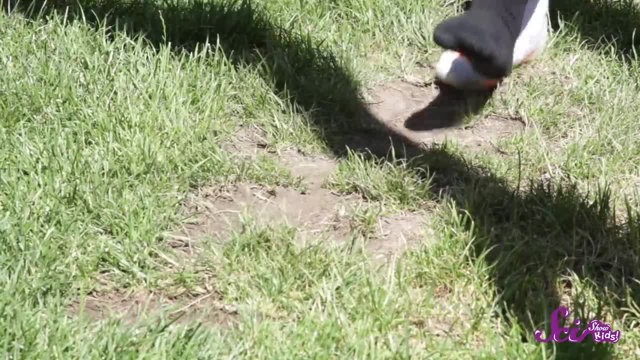 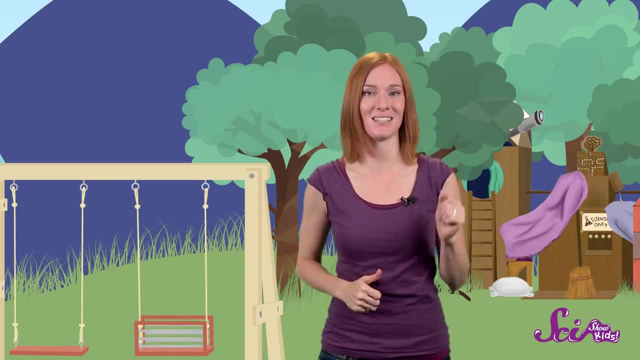 to a complete stop. You can even create more friction. If you drag your feet on the ground, you can help yourself stop faster. Now do you know another place on the playground where friction is at work? The slide. Gravity pulls you down the slide, but friction between you and the slide slows you down. 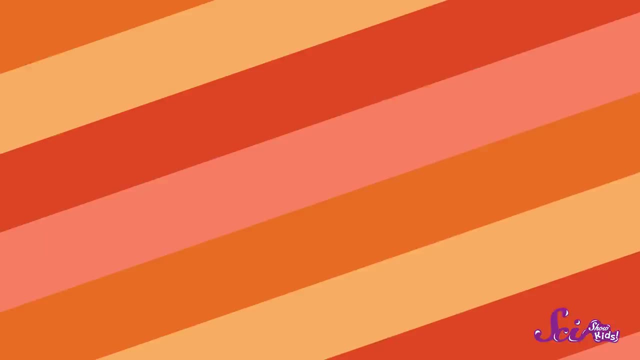 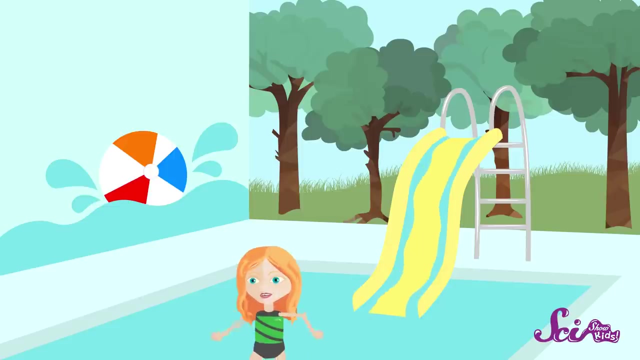 So it lets you go at a fun but not scary speed. But have you ever been on a water slide? The reason you can go down so much faster on a water slide is because water reduces or takes away some of the friction between 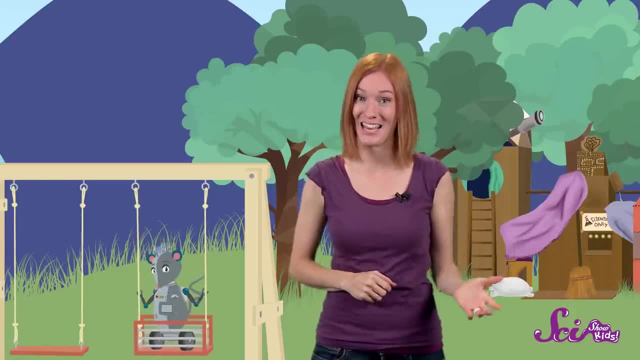 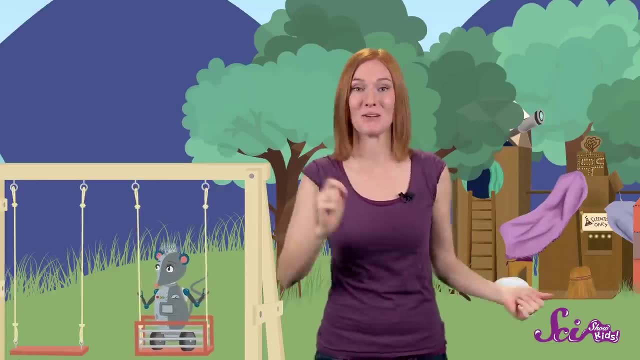 you and the slide. Good thing, there's a nice big pool of water for you to land in at the bottom. So now you know how forces work at the playground And everywhere else. Now go outside and get your body in motion and see what forces you discover. 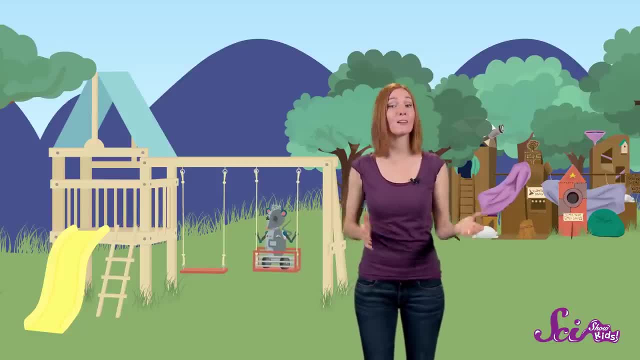 Thanks for joining me on SciShow Kids. If there's something you'd like to learn more about, let us know by leaving a comment or emailing us at kids at the scishow dot com. Thanks, guys, and we'll see you next time on SciShow Kids. Kids at the Fork.